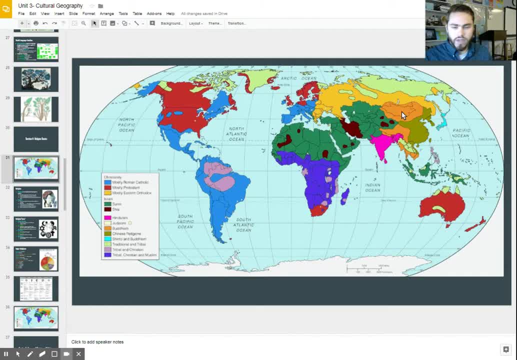 So here are, as you can see, the different religions of the world and where they are located, And I want you to take a minute and see if you can pick out any patterns. First of all, use the legend to help you tell what religions are represented by what color on the map, and also where those religions are located and where they share common religions and where they have different religions and where those boundaries are at. 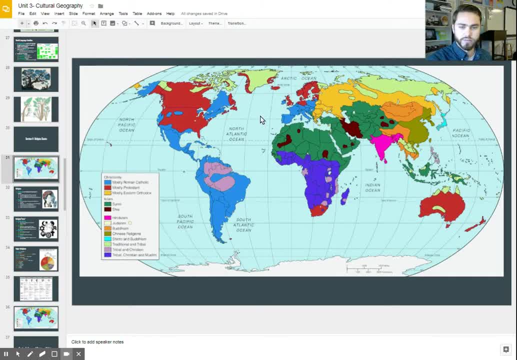 All right. So one of the patterns I want you to notice is is both Christianity and Islam which are largest religions and most widespread, and see where those are located. These three types- Roman Catholic, Protestant, Eastern Orthodox- are your main three that are located throughout the world for Christianity and then Islam. 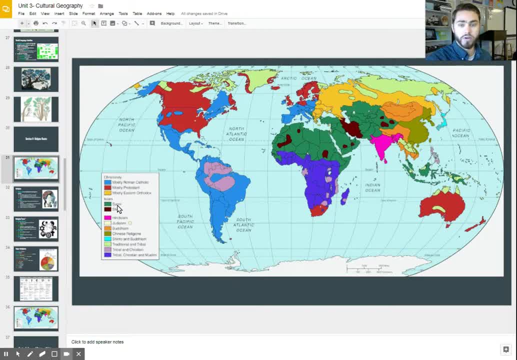 There are multiple kinds as well, But the main two Branches are Sunni and Shia Muslims, and you can see those are predominantly located in the Middle East and North Africa, here shaded in green and the dark red, And there are some other places as well. 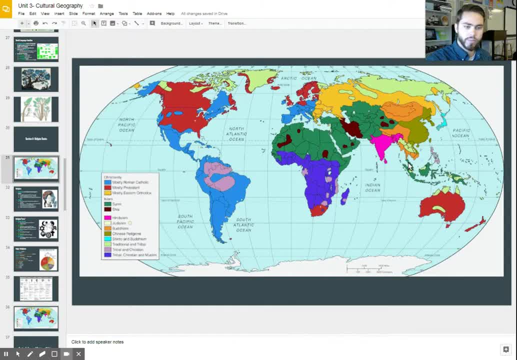 Notice here in Indonesia and parts of Papua New Guinea they are predominantly Muslim as well, And you can see where Christianity is. its origins obviously in the Middle East here, but really took hold in Western Europe especially. Hey, Mr Kelly. 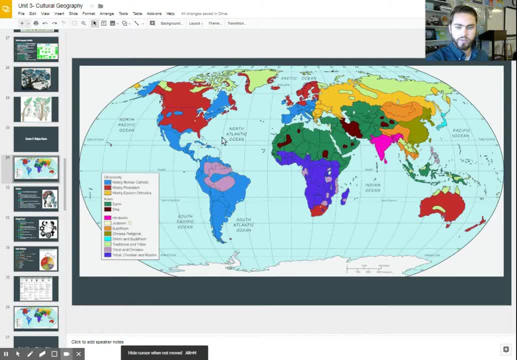 Hey, how's it going? All right, And you see where Catholic Christianity is mostly located here in Western Europe and also in North and South America, especially here in Central America, the Caribbean and South America. It's predominantly located as well, And I want you to be thinking about where that spread may have come from as well. 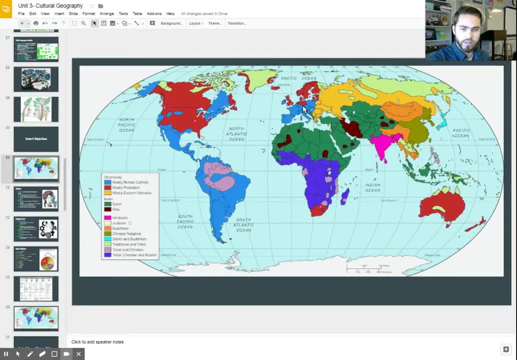 As for Protestantism, it started in Germany, where it originated, and we can see how that's transformed different regions around the world, especially in southern Europe and parts of North America, And we form栶Р milhões as such in places such to characteristics of in South Africa and northern Europe, but also places such as South Africa, Australia, New Zealand and other places around the West. 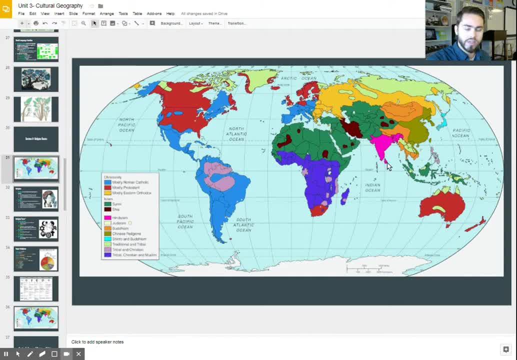 We can see how that is able to transform the different places around the world. I want you to focus on and notice where they are- South Asia as well- as I want you to focus on Buddhism, which is mostly in Eastern Asia, here in orange as well. and finally, Judaism- all right for the Jewish. 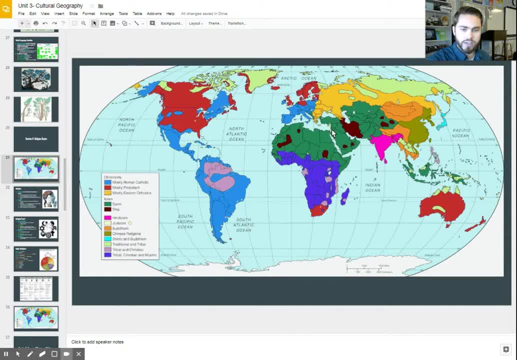 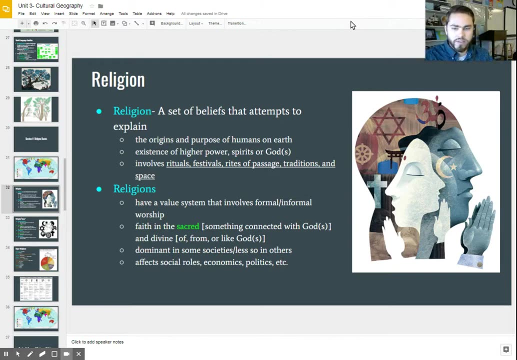 population here, where predominantly located in Israel, although there are large populations in Europe and North America as well. so let's get into what religion is first of all. religion is, as it says here, a set of beliefs, and it's basically trying to explain things that are that cannot be known for sure, right? 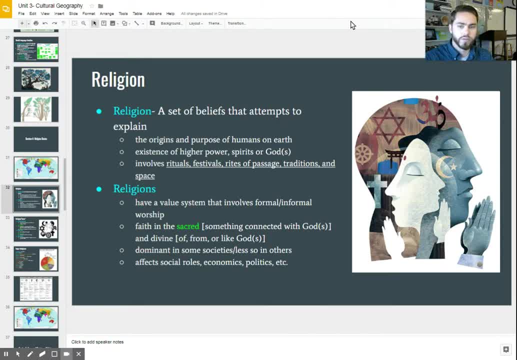 so, such as such things as the origin of the universe. you know where mankind, mankind came from, what our purpose as human beings are on earth. are there higher beings, spirits, gods, things of that nature? and they usually involve these things you see here, such as rituals. all right, that could be in. 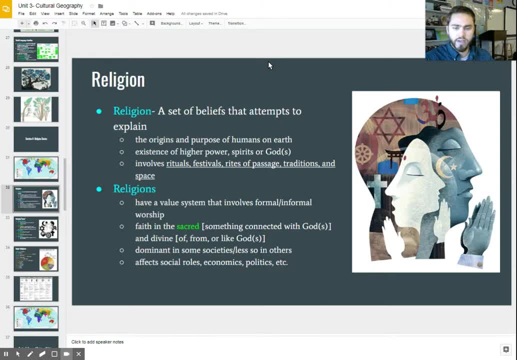 Christianity, such as taking communion or being baptized, and you know Judaism. you have the bat mitzvah, the rite of passage, for you know men in that culture become first. you need boys in that culture becoming men. in Islam you have the pilgrimage to Mecca. these are all types of rituals that are performed for one of 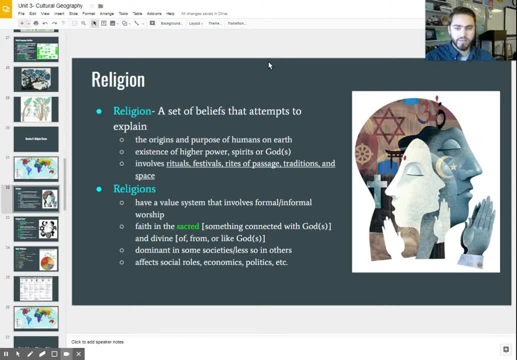 the, the common traditions in the world, and while these are not part of any religion or religion, they are actually part of a particular religion, a particular religion or religion that is considered to be a religion in the world, and it is a symbol of that particular religion and it has some type of meaning attached to as well. it's more than just. 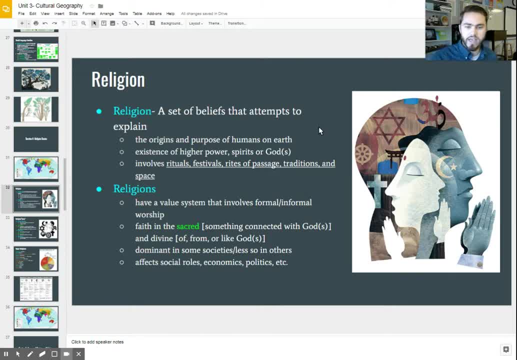 the actual act. it's a sign, it's a symbol of what those acts mean to that particular religion, and they vary, of course, from religion to religion. but these are heavily involved in traditions and you know holidays and ways of life. you can see the traditions of Christianity intertwined in our day-to-day lives. 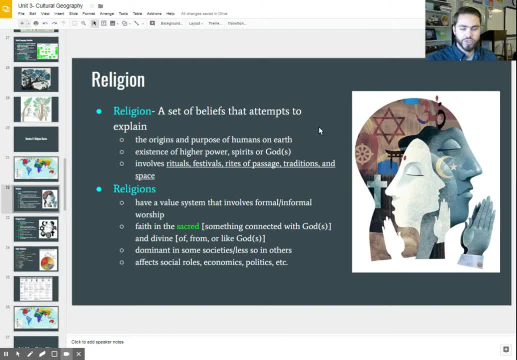 You know, here right now, we are getting ready soon for the Christmas tradition, which is, of course, a Christian holiday, And you can see how that is playing out in our society as well. So obviously we can see how big religions can affect our day-to-day lives. 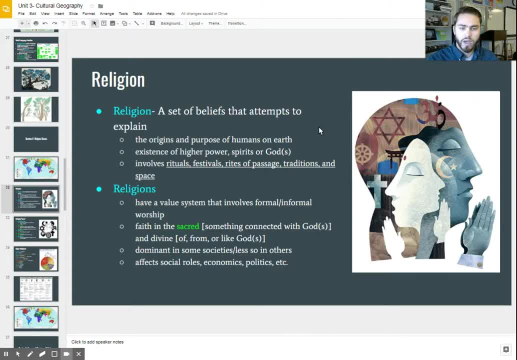 And this is true not just in the US, of course, but around the world, in other Christian societies, but also in non-Christian societies, where you have other holidays and traditions coming soon. We know Judaism. they have Hanukkah and other religions. 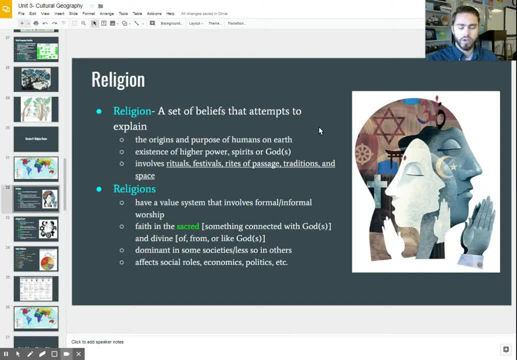 They're celebrating around this time of year as well, And we'll take a greater look at that later on, But it's heavily tradition-based. It's passed down from generation to generation And they're taught the same traditions in each of their family units and tribes. 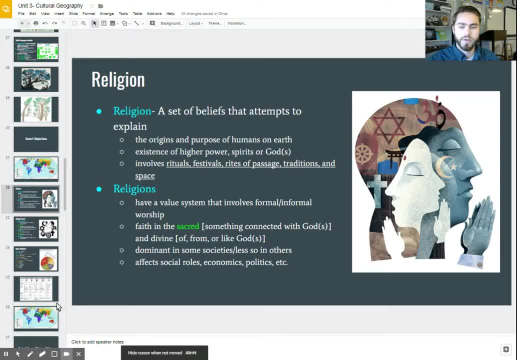 and things of that nature, All right other things that religions have. All religions have a value system, Things that they hold as being important. These are oftentimes written into their holy scripture or books. They're written into their specific church doctrines. 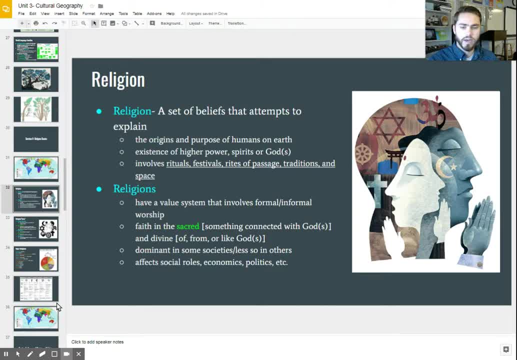 And they're also informally practiced by all the members in that particular religion. You have different things, behaviors that are deemed more worthy, And usually they are attempts. They're attempts to make people fall in line with things in society that are deemed good. 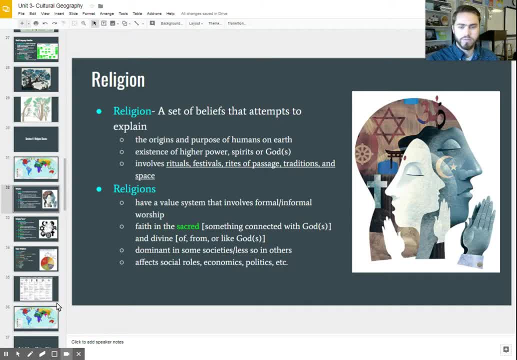 So it's good things like taking care of your neighbor, helping the poor or feeding the hungry, or being kind to one another. These are types of values that many religions have and place an emphasis on Now. many religions also have a place of value on things that are what they deem sacred. 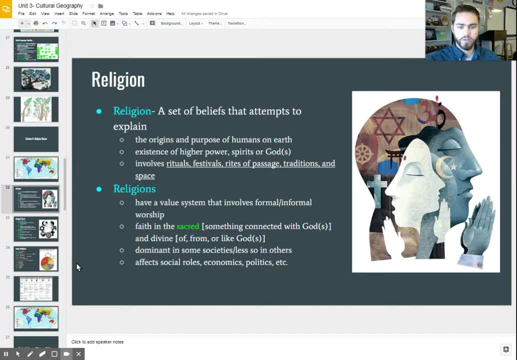 or connected with God. This could be a physical item, such as a cross. It could be a menorah In Judaism. it could be a holy text such as the Quran in Islam. You know, things that are deemed connected with God are what we call sacred. 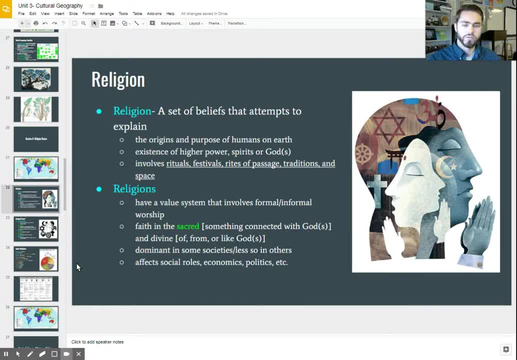 And these things are held in higher regard or divine, And some things are considered actually from God or a way in which God has connected to the spiritual world, or multiple gods- in some religions It could be spirits, But it's something that's connected with the spiritual world. 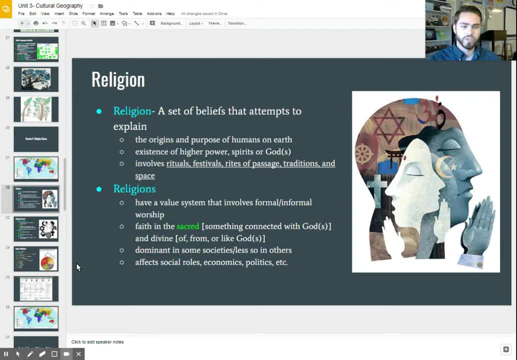 It's something tangible we can see or touch, And so in some societies these are very important things. In others, you know they're less, so You can see a more religious society, based on their laws or value systems, or less. 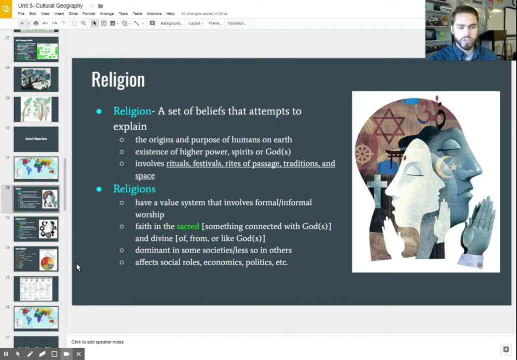 or more religious or less religious, depending on what religion is dominant in that area and how strict they are of followers. And it affects not only people's lives day to day but also their social roles, what jobs they have, Holidays, of course. 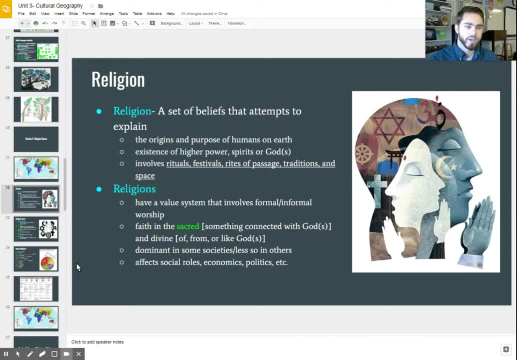 We talked about, it could be a political issue. We see it all the time in the US, you know. you know religion as being a political issue, And it's even more so in many other countries. All right, A couple of isms that you need to know. 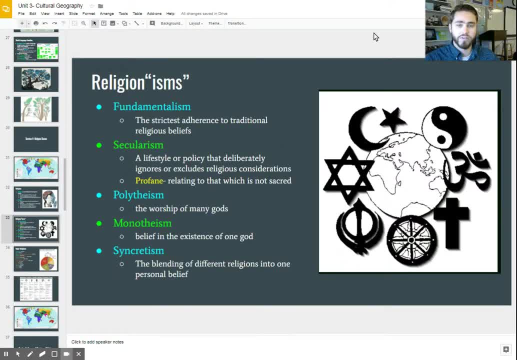 Number one: fundamentalism. This is where you have a very strict adherence to your religion and its beliefs. You know, these are the people you think of that never miss a particular religious event. They always follow all the rules of that society. 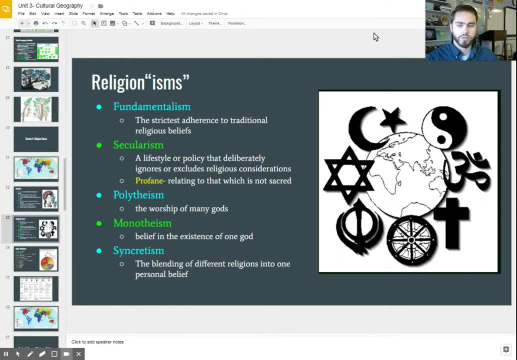 Maybe in Muslim culture you know that they don't eat pork or don't drink alcohol or always follow the teachings of the Koran. These are very strict, fundamentalist by the book type of followers, And that's as opposed to a more secular view where you have a lifestyle that's less adhered to. 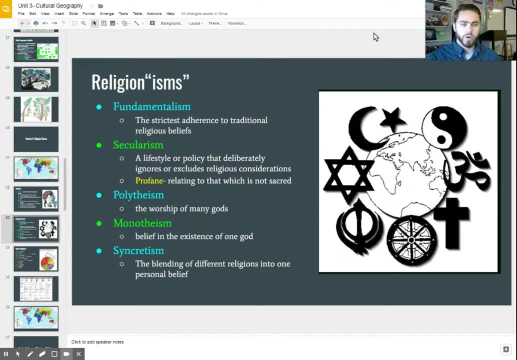 whatever religion that you are, Basically, you don't necessarily follow all the rules, or or maybe you only go to church a few times. It doesn't make you less necessarily- It's just how- of that particular religion. It just is saying that you don't follow it to the strictest of the law, of whatever religion that you're talking about. 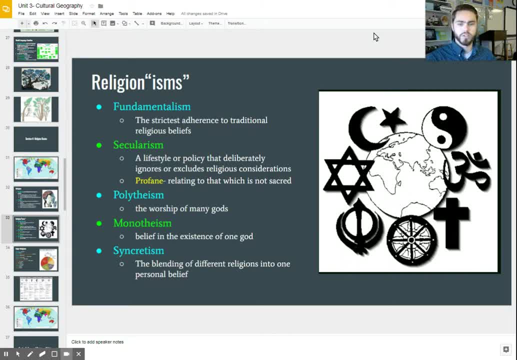 And sometimes this is to the degree where you are nonreligious- And we're going to talk about that's one of the fastest growing Belief systems out there- is that you are not concerned with religious aspects and you live a more secular lifestyle. These are things that are not considered sacred or are part of that particular religion. 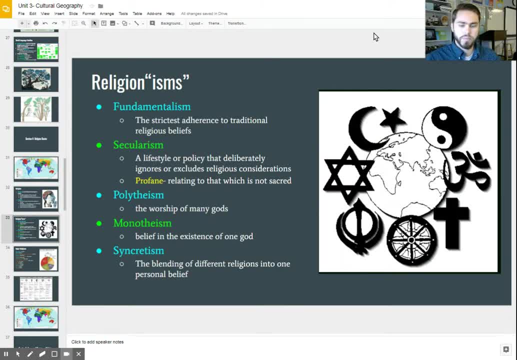 Also a couple other types of isms that you may have heard of before. It's poly and monotheism, And that's just the belief system of different religions and how many gods there are. polytheism- Poly meaning many, That there are multiple gods in that particular religion. 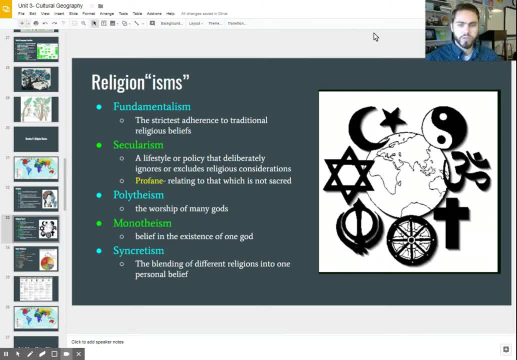 And they usually have some type of of specific job or purpose. Those individual gods do you know? for example, in Hinduism you have different gods and they all have a specific purpose, such as you know. they're the particular god of forgiveness or love, or so on and so forth. 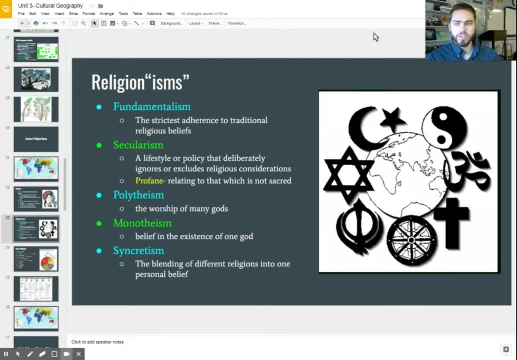 Whereas in monotheism there is one god in that particular religion. These are religions such as Islam or Christianity, Judaism. These are monotheistic religions where there's one all powerful God, and they usually handle all aspects of godliness. 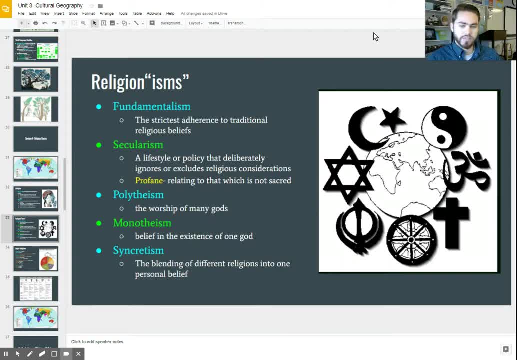 All right, And finally, the last ism we're going to talk about is syncretism, And syncretism is just when you start seeing the combination of multiple religions into one personal belief system. that is typically held, And the number one way in which you see syncretism around the world is through Buddhism. 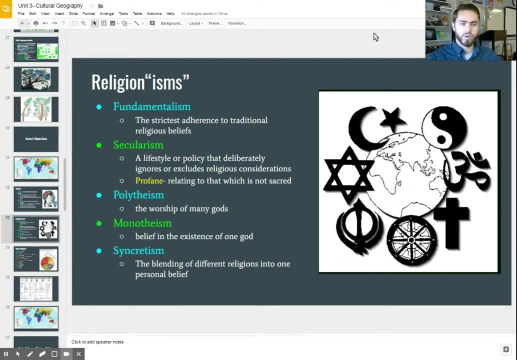 So Buddhism does not necessarily particularly push forward any one particular god. Many people live a Buddhist lifestyle because it's basically a way of life, a way to live according to Buddhism, And you can have really any other type of god or gods as your personal belief. 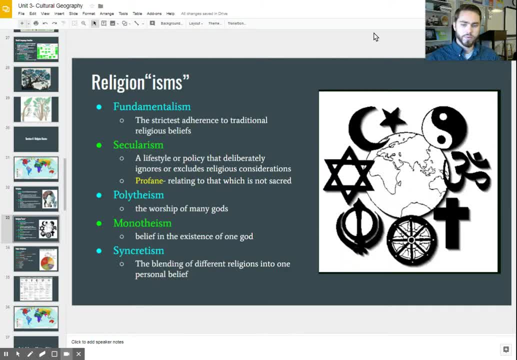 And Buddhism does not discriminate in that sense. And so many people have combined Buddhism and Islam, Buddhism and Christianity, Buddhism and many other different types of religions to form a syncretic religion Where it's blended their different beliefs. All right, Real quick. 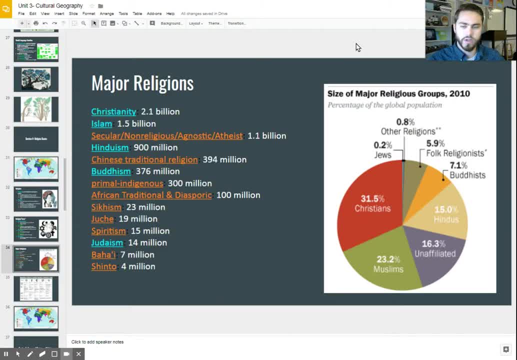 Here are the numbers that we see around the world of Christianity. Islam, Hinduism, Buddhism and Judaism are the main ones we're going to focus on, So make sure you pay attention to the order there and how many adherents you see, Christianity being the number one religion in the world. 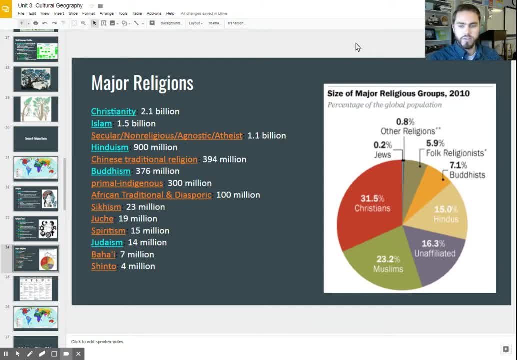 However, Islam is still the fastest growing And so soon they say, Islam is going to have pretty comparable numbers, Probably in the next century, by 2100 or so they're going to be about even with Christianity in terms of total followers around the world.